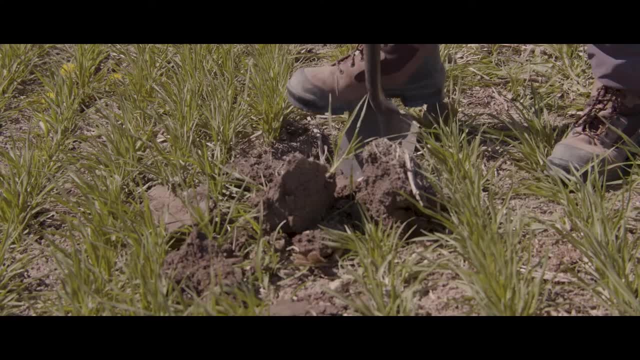 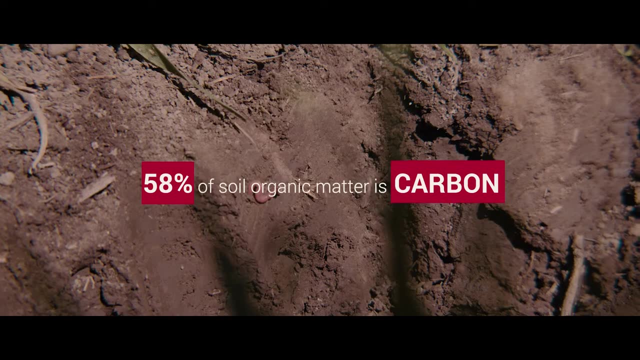 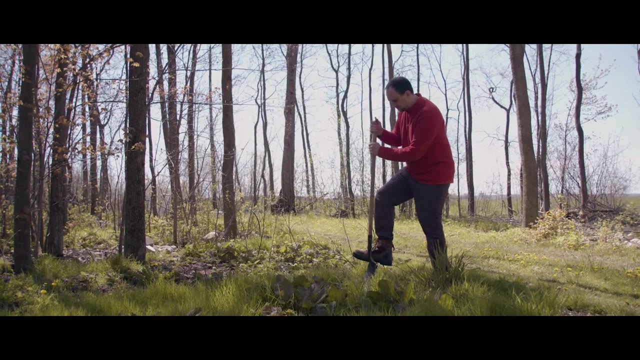 So you can think of it as decayed material in various stages of decomposition. Roughly 58% of that is going to be the organic carbon that is found in the soil. In many cases, the bigger root of carbon input into soils is through dead roots and what we call root exudates. 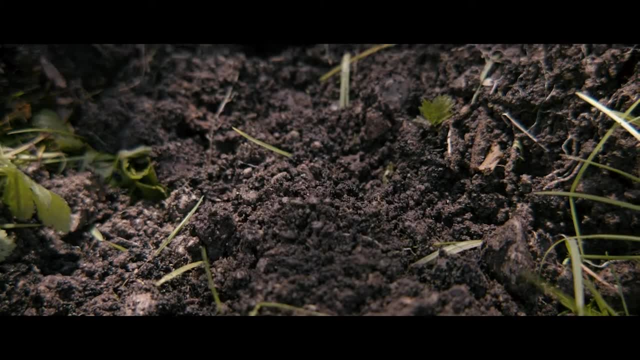 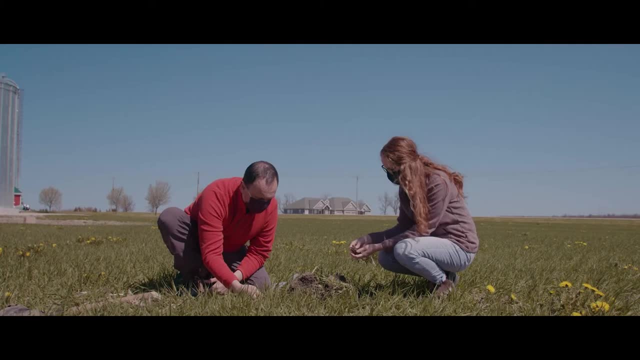 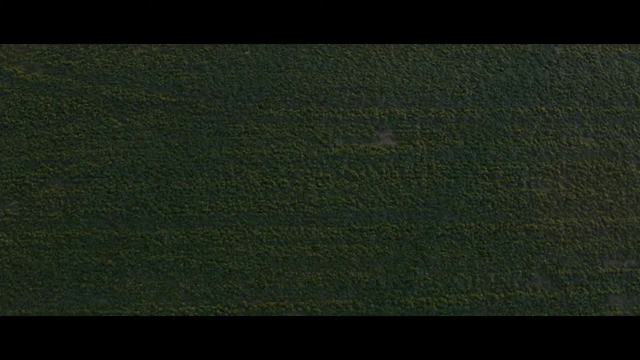 So organic compounds that are released by the roots as they are alive. We're really trying to follow best management practices that are laid out by our researchers and government professionals. We focus on three main pillars: The first, which is reducing our tillage and general soil disturbances. 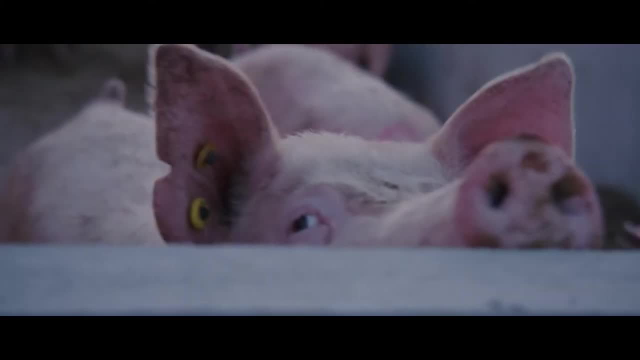 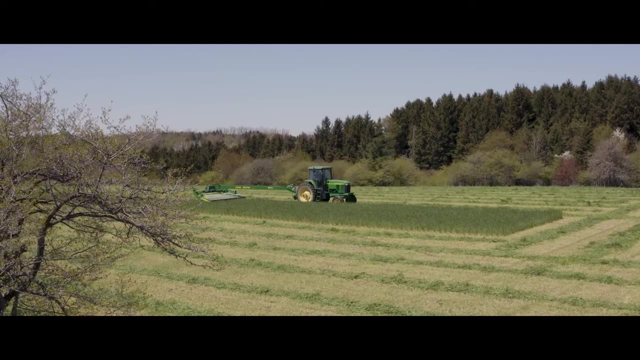 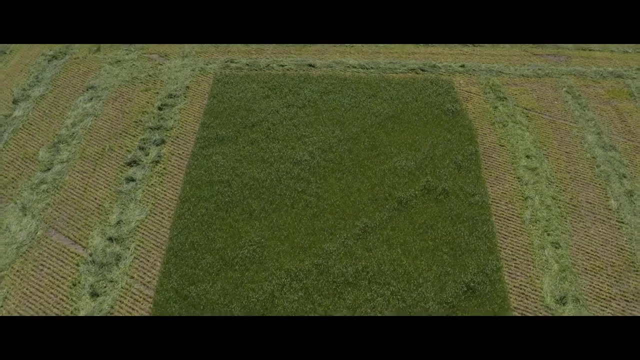 The second being integrating livestock into our cropping systems And the third being enhancing diversity at every aspect of our farm system, Both on cash crops and cover crops, Growing everything from the traditional corn, soybeans and wheat right on through to triticale peas, alfalfa. 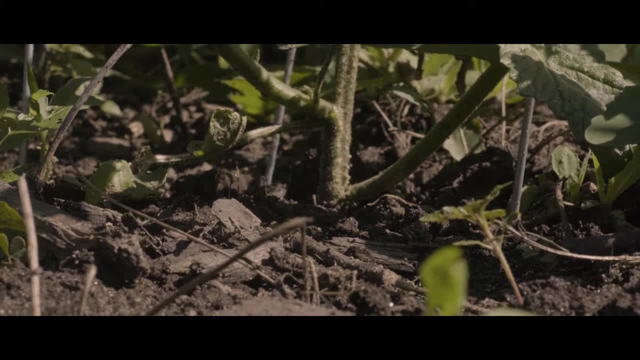 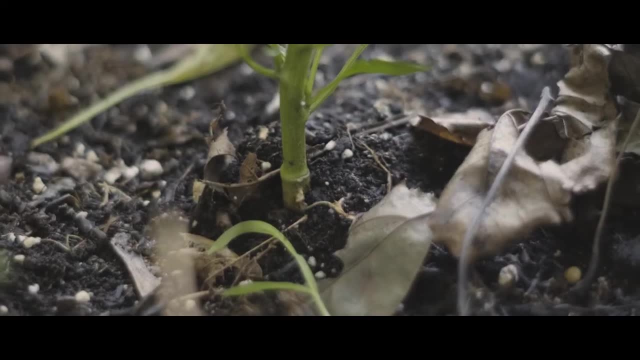 That's why it's a win-win really. We can sequester atmospheric carbon and we can actually put it into the ground and benefit the resiliency of our soils. So it's not a trade-off. it's kind of a both-and approach we can have here. 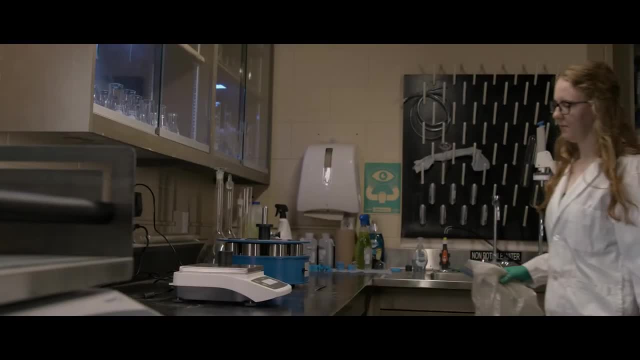 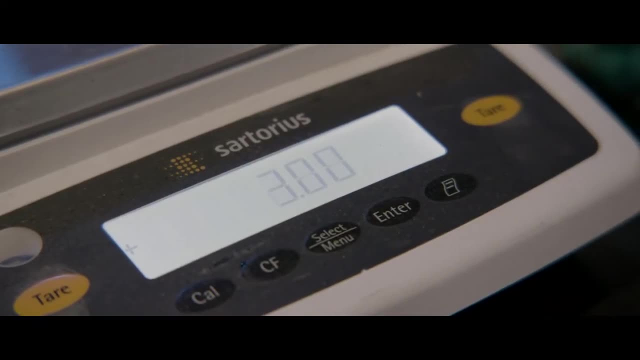 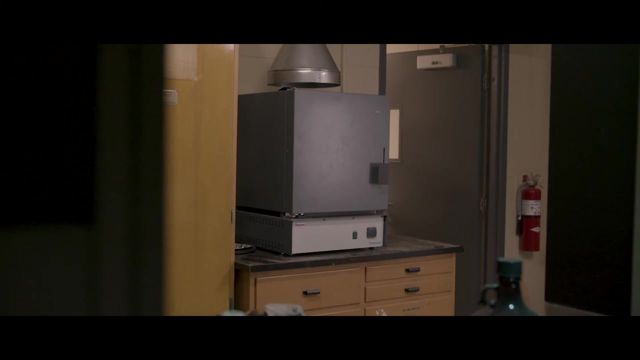 So my master's research project is focused on soil organic matter and soil health indicators. Active Carbon is looking at the available carbon that's in the soil and it's available for microbes to utilize and it's a really great measure of soil health because of that. 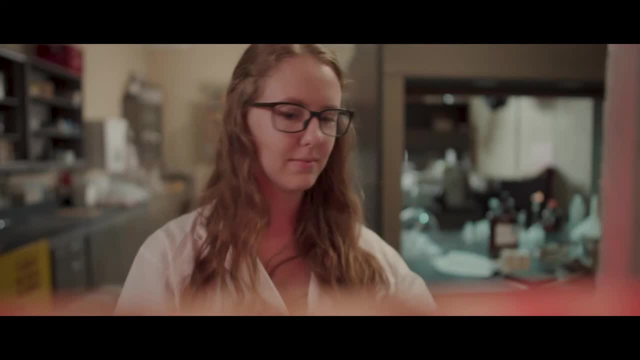 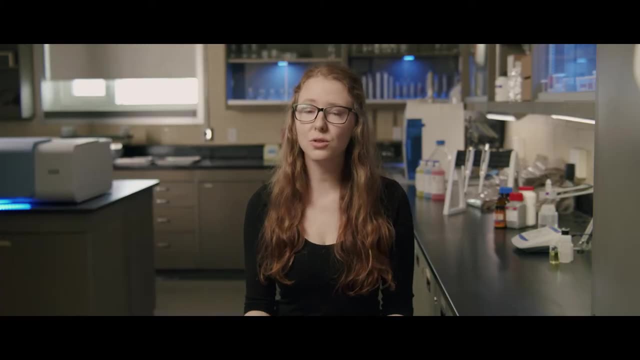 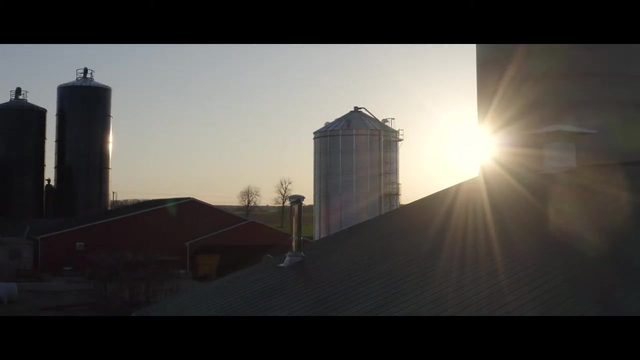 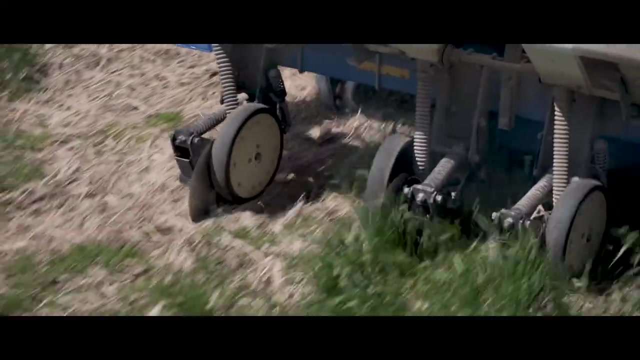 One of the big research drives is to see how stable organic matter is to decomposition. It can be easier to lose some of the soil- carbon rather than store it. Some of the best management practices that help to store carbon in the soil include reducing tillage, planting cover crops, diverse crop rotations. 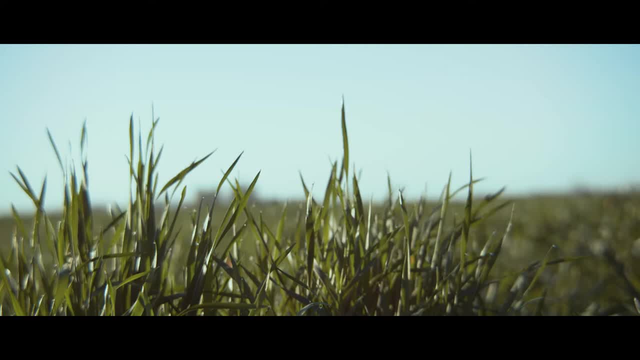 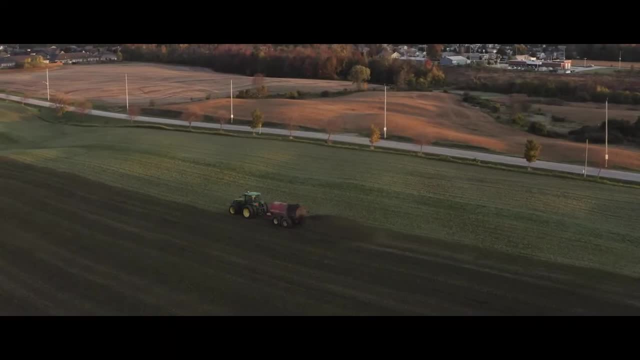 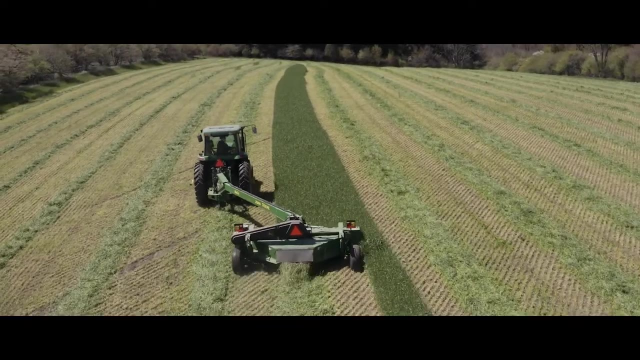 making sure the soil is covered year-round with a cover crop. So having those best management practices really relates to healthy soil, which in turn helps to reduce the overall effect of climate change. The benefits of us integrating these practices into our system are quite limitless.